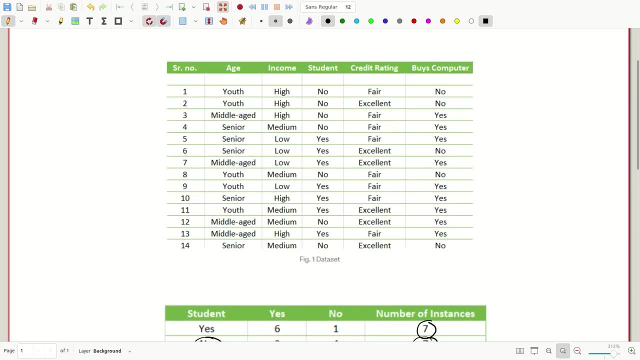 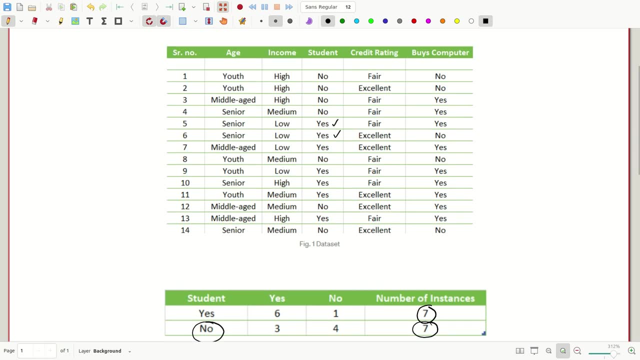 for when the student was no, when the candidate was not a student. Out of these seven values of yes, that are one, two, three, four, five, six and seven, six times the individual has bought the computer. The class of the biased computers is yes: One, two, three, four, five, six. So we have 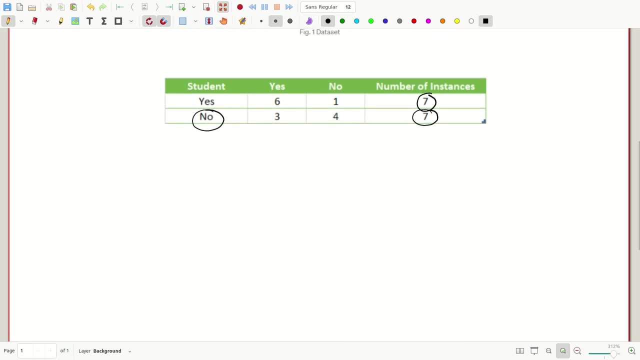 written these values in the form of the table. Let's do the mathematical calculation now. Well, Gini value: while the student is equal to yes, The total instances while the student was yes are seven, and out of these seven, six times the person has biased computer. yes, class. Square it down. 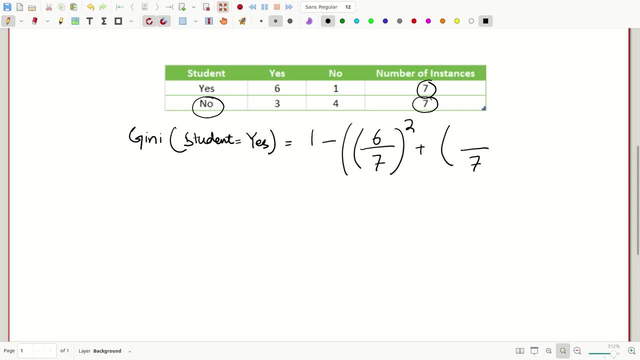 while out of these seven instances of yes, only one time the class of the biased computer is no. Well, the value as the result of this mathematical calculation is 0.246.. Now let's calculate the Gini value while the student was no. So the total instances when the student was no are nine, and out of these, sorry. 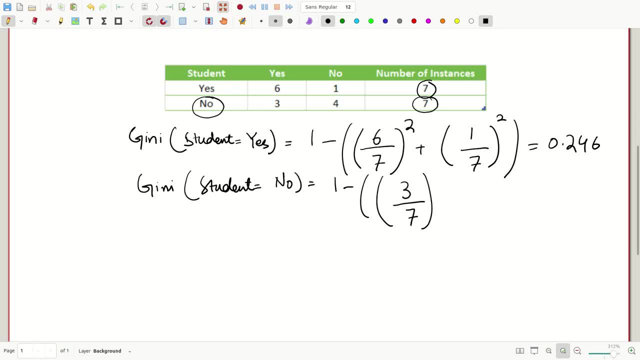 seven values, and out of these seven values, three times the biased computer class is yes, While four times the biased computer class and after doing the math we'll get 0.489.. Now we want to calculate the Gini index of this student feature, So we will have to sum both these values. We will have to get 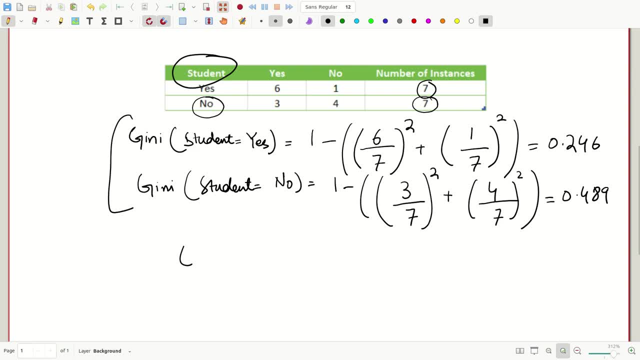 the weighted sum, In fact, right So the Gini index, while the for student feature of this data set are 0.246 plus 0.489, and since we are going to calculate the weighted sum, well, seven instances of student yes out of 14.. this vedere, 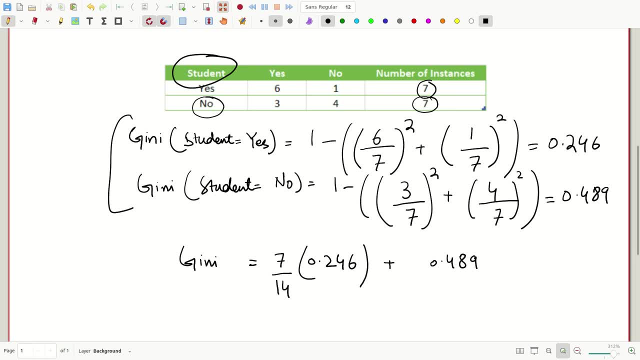 of this, uh, while the student was yes. similarly, 7 out of 14 is the weight of the student. no value. and after getting the, after having the mathematics, well, the final value is 0.367, right 0.367. so this is the genie value, the gene index value of the feature student. now we have only last. 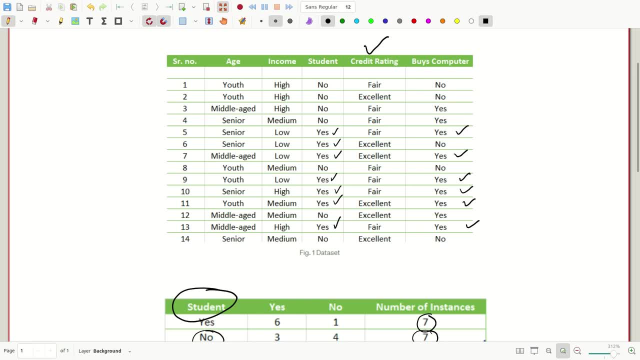 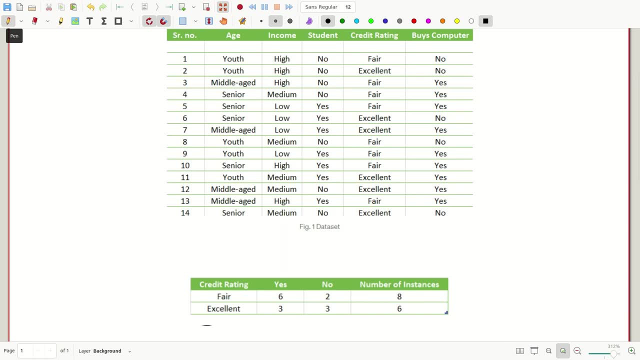 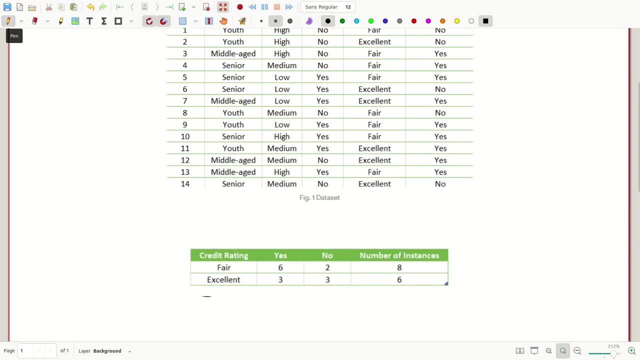 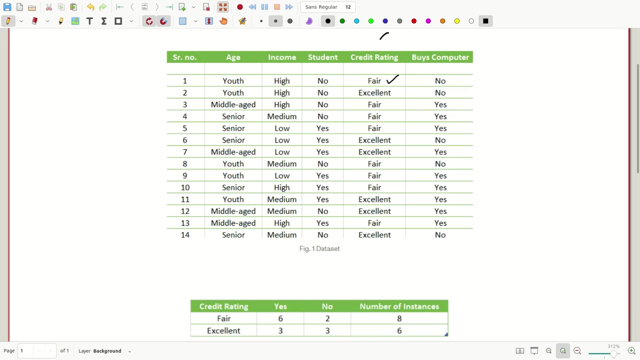 feature remaining, that is a credit. we will do the same for it. so let's bring in the table of the credit rating. well, if you look at the data set again, let me re-explain it. well, the credit rating genie index value has to be calculated now and it has total of eight fair values: one, two, three, four, five, six, seven, eight and six. 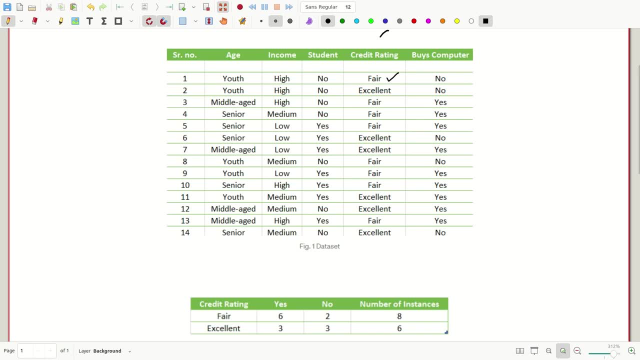 excellent values and out of these eight fair values we have six times: yes, class right one, two, three, four, five, six, seven, eight. and out of these eight fair values we have six times- sorry, it's not included this excellent one- six times we have yes, class of the bias computer. 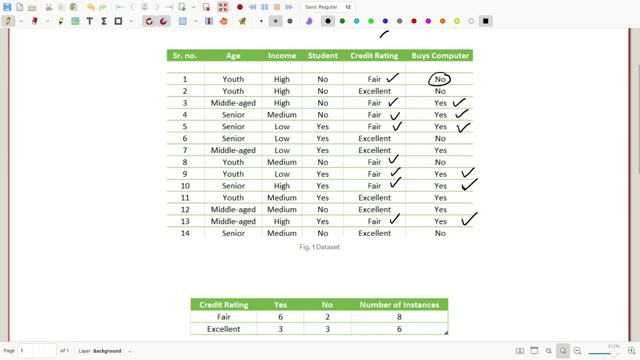 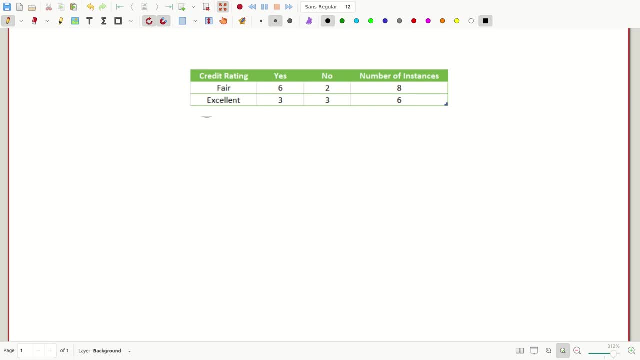 and two times no class. so we have summarized these values in this, in the form of this table. so let's calculate the gene index value while the credit rating is equal to fair, one minus well, total of eight values of the fair well, the credit rating one when the credit rating was fair. 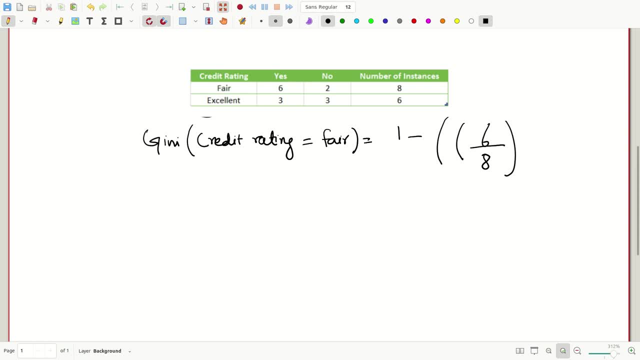 and six. out of these eight values, we have six uh times the bias computer yes class and two times no class. well, after doing the mathematical calculation, we will get 0.375. similarly, while the credit rating is equal to excellent, one minus three out of six whole square. 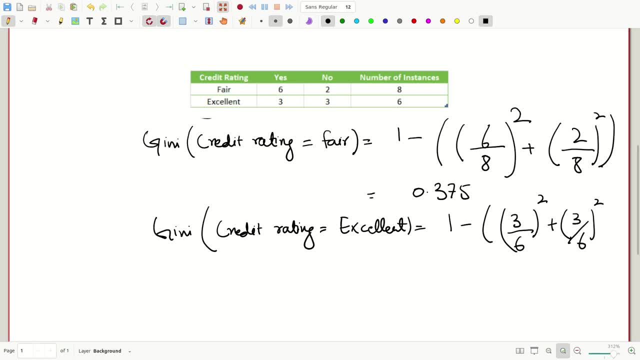 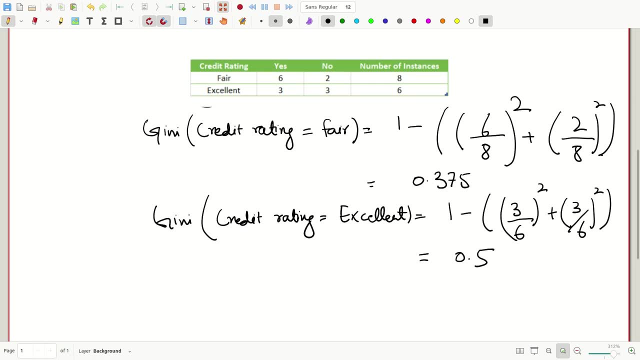 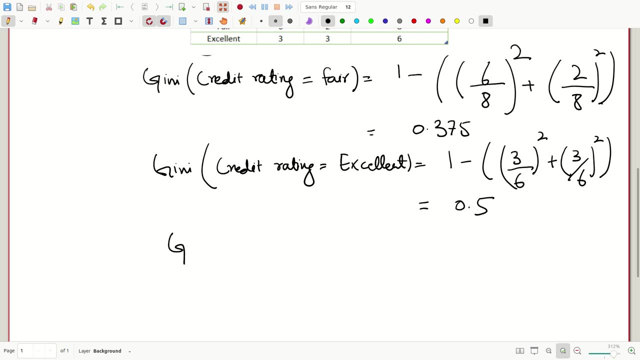 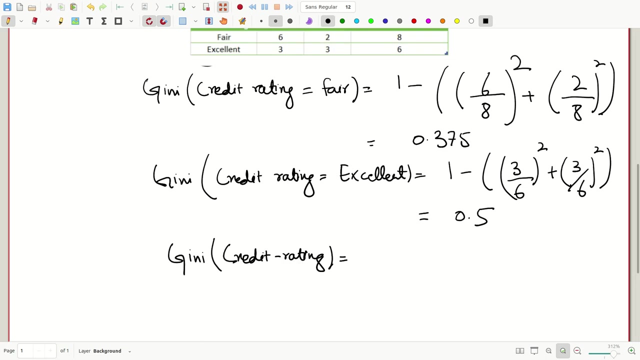 plus three out of six whole square. well, that would be equal to 0.5. now we want to have the weighted sum of both these values to get the genie value of the entire feature, that is, credit rating. that would be equal to well, eight times. we have value of fair and the total. 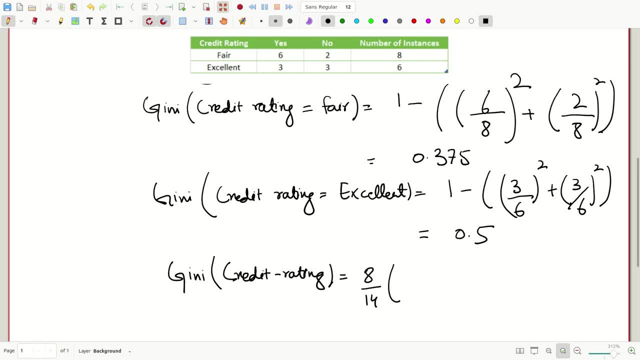 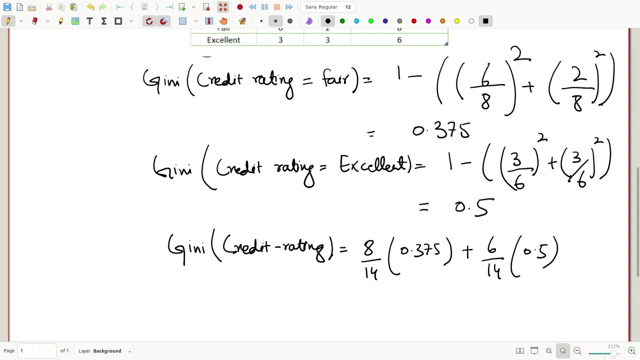 values are 14 and by 14 is the weight of this fair. 0.375 plus 6 by 14 is the weight of the excellent, and the gene value individually calculated is equal to 0.5, so 0.428 is the value. 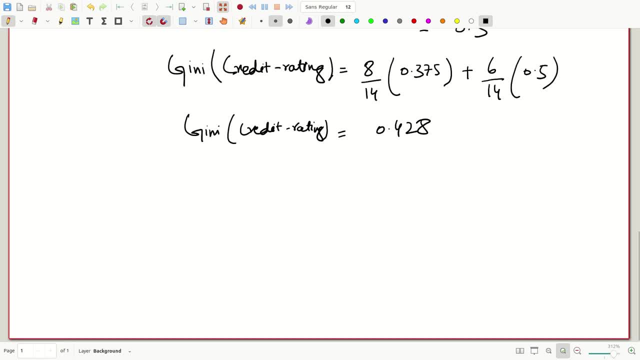 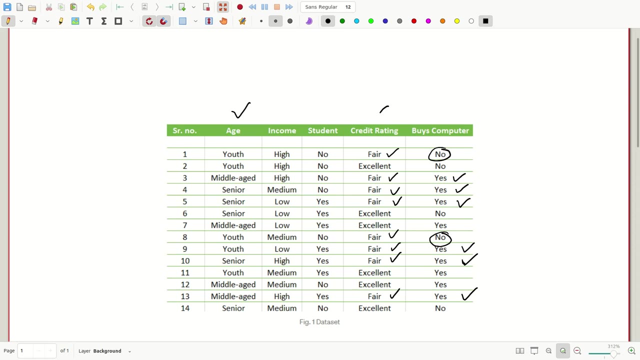 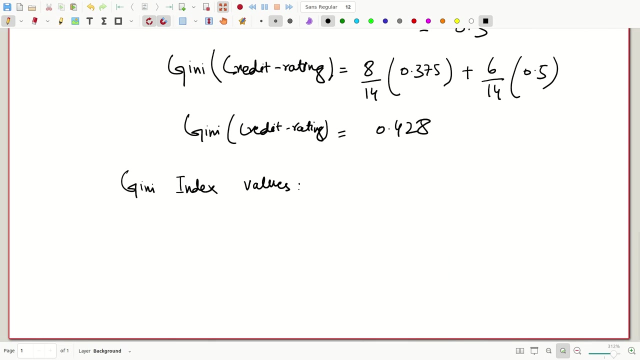 of the genie value of the credit rating. so let's have the comparison of the gene index values now. so if you look at the gene index value of all these four features or parameters of the data set, well, we have one person who has an evidence of this from the last one. 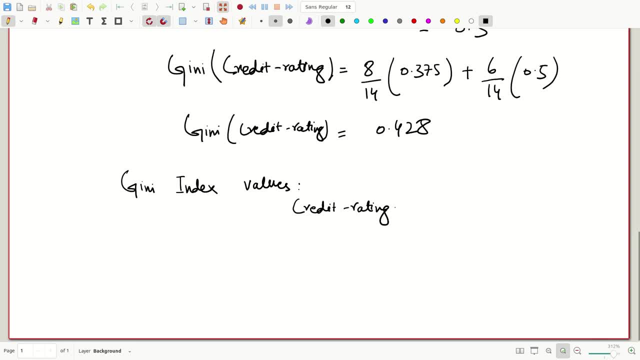 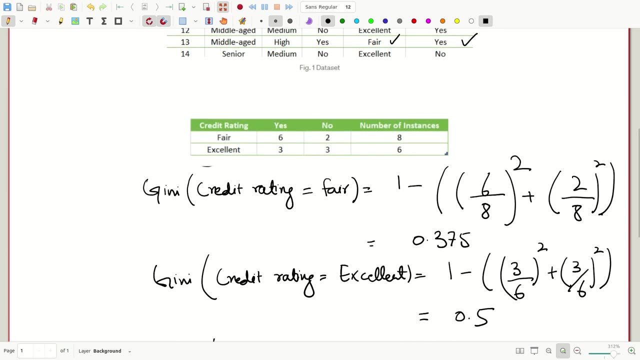